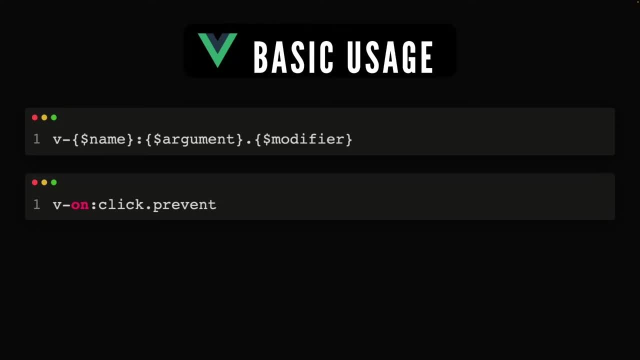 comes the directive modifier. Now it's important to note early on that not all directives take in arguments or have modifiers. but in our example we're using the v on directive that's going to add an event listener to our element, onClick, and onClick will also use the prevent modifier. 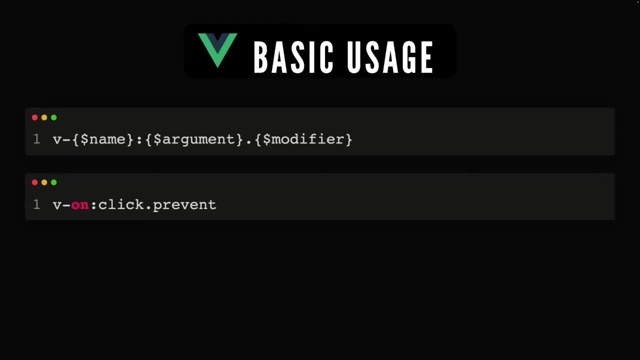 So in the JavaScript context, wherever I see prevent, I typically think prevent default. right, and that's exactly what's happening here. I'll click, it's going to run prevent default for you. and then, lastly, if that directive takes in a value, that's passed in with the equal sign and it's wrapped in quotation marks, so once more in our 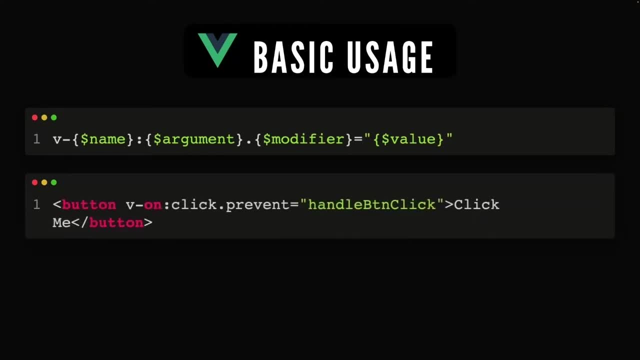 example, we're going to add this to a button on our page that will tell view on click of this button: prevent default first and then run a function called handle button click. the last thing to point out is that some directives do have a shorthand version, so in our case we can replace. 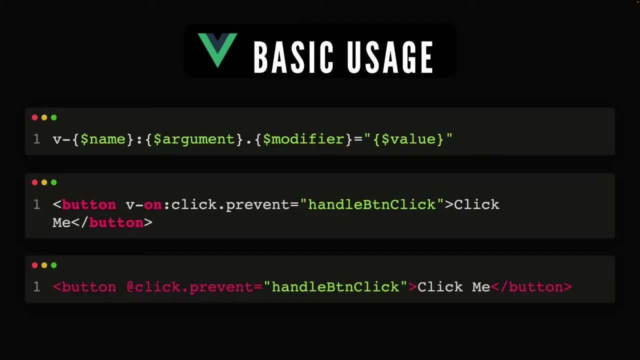 v on and colon with the add symbol in front of the click right there, and all i'd say in terms of that is just be consistent. if you're going to use it in one place for that particular directive, then use it wherever you use that directive. okay, now we're going to take a closer look. 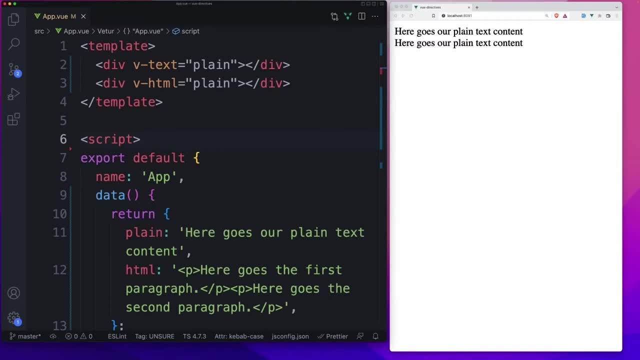 at some of the built-in directives. we're going to start off with vtext and vhtml. now, these two are very similar. both of them will assign content to an element, so things in the example in front of you here we've got two data properties: a plain property and then an html property. 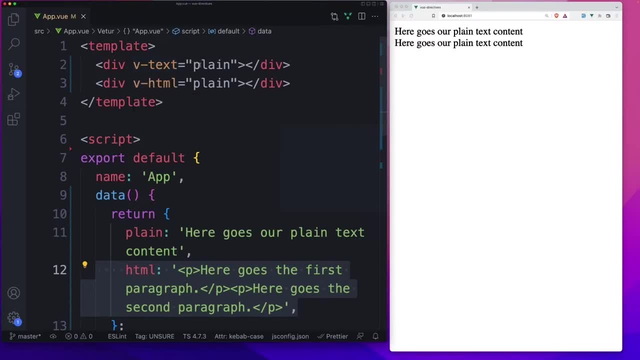 and right now i'm assigning plain, using vtext for the first of and vhtml for the second. now you won't see any difference because it is just plain text. but if we change the plane to be html, now you'll see the difference. right: vtext sets the elements text content property. vhtml sets the. 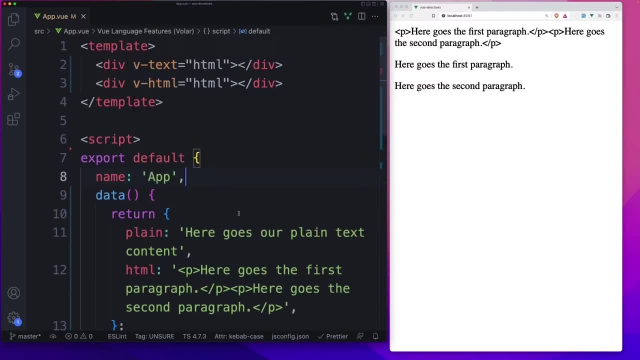 elements inner html property, and that means anything that you assign through v html is going to be treated as html. so you've got to be careful, you've got to make sure that you can trust the content and you're going to be able to get the content that you're going to want and you're going. 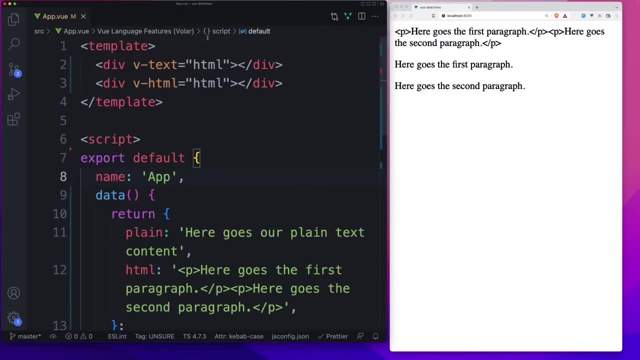 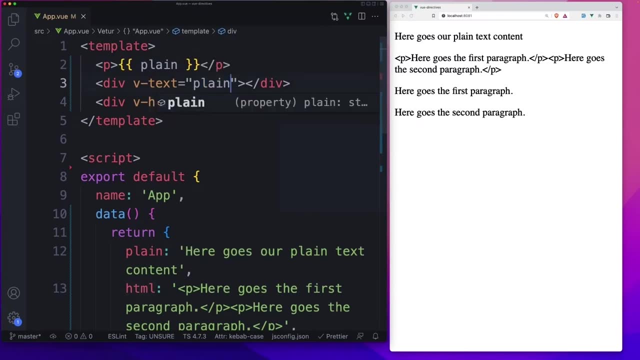 to be able to get the content, but it also means because of the way vtex works. really you're better off if you only had plain text doing something like this, because right now, between the first paragraph and that, right there, there's no difference in the outcome side of these two. 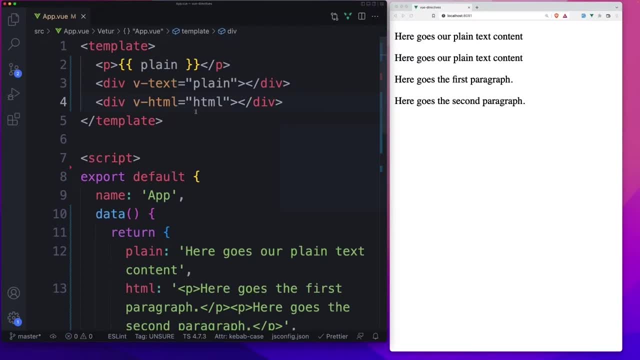 i don't really use vtex at all. i'll use vhtml if i have html coming back from an api. otherwise i just use that format right over there. now be aware that you can't have anything inside of the elements for either vtex or vhtml, so we couldn't do that. 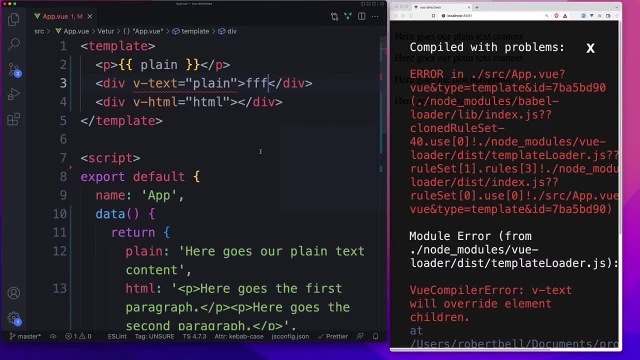 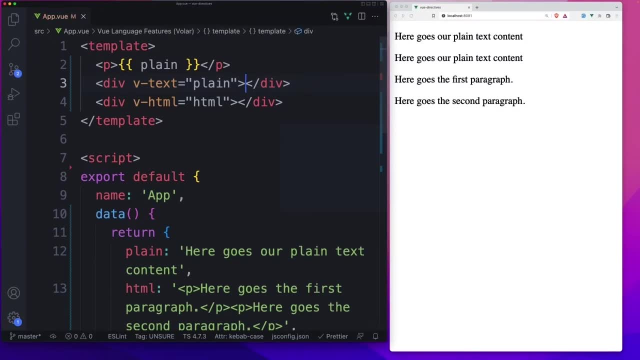 let's try and do that, and view is not going to lie. and that's because when view sets the content for these elements using vtex or vhtml, it'll override any of the child elements inside of it. now there's no shorthand for these directives, so it's always going to be with the prefix v dash. so 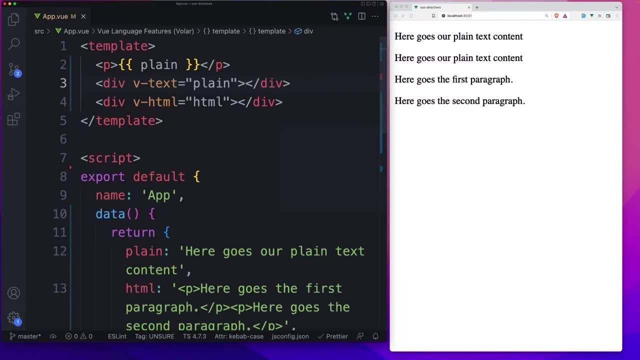 vtex, vhtml. and the last thing to point out about this is, when it comes to vhtml, be careful with your styling. so we can't apply scope styles. so right now we've got our paragraph tag on there. let's say we wanted that to be say red. so if we apply our styles globally as we have, 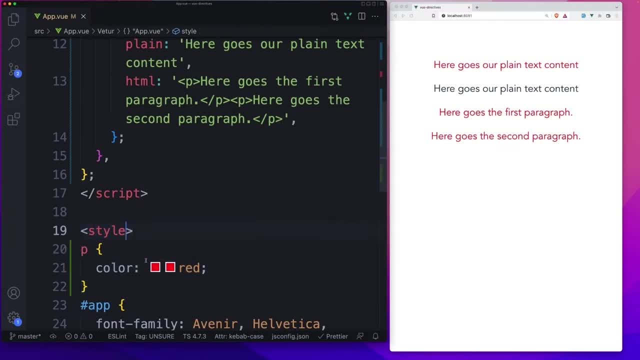 as we have right there with that style tag, that's going to work fine. if we try and make it scoped now, suddenly it doesn't work anymore. so the paragraph tags coming in through our vhtml: they remain black. if you do need to apply css only to that particular component. 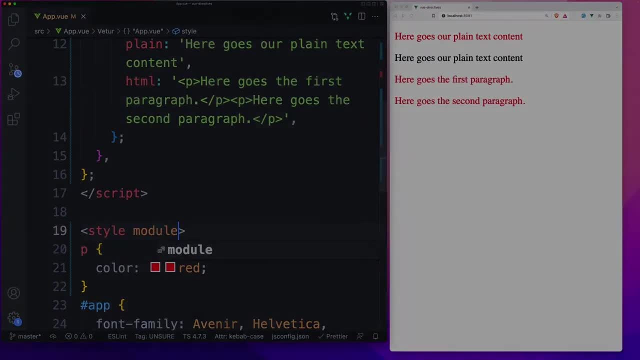 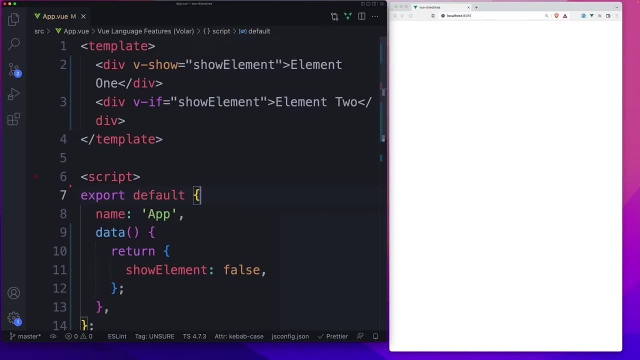 then you can use css modules. next we're going to look at v show, v if, v else and v else if. all four of these directives deal with showing or hiding content. v show and v if are the two that control showing or hiding the content, so in other words, both these. 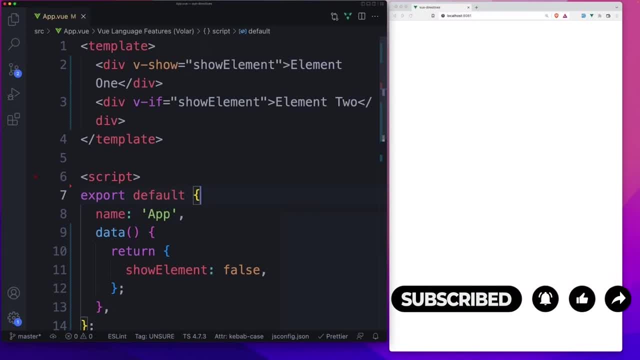 directives will take in some sort of statement and, based on whether it's true or false, will show or hide that content for you. v else and v else if just allow you to extend your vf and if you're used to javascript writing, and if else else if it's the same sort of thing. so in the example in, 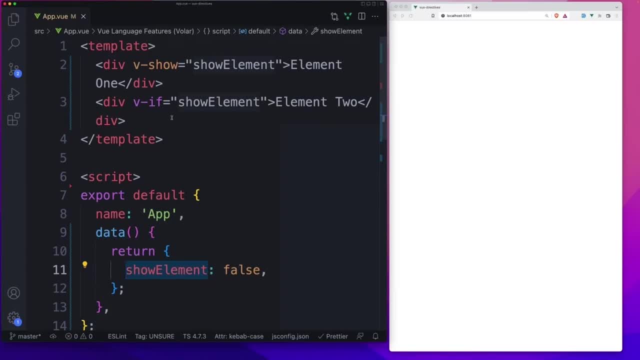 front of us. i've got a data property show element and that's set to false, so we don't need to change that. so we're just going to use v show and v if for element one and v if for element two. now here's the difference between the two: v show will still render the element on the page. 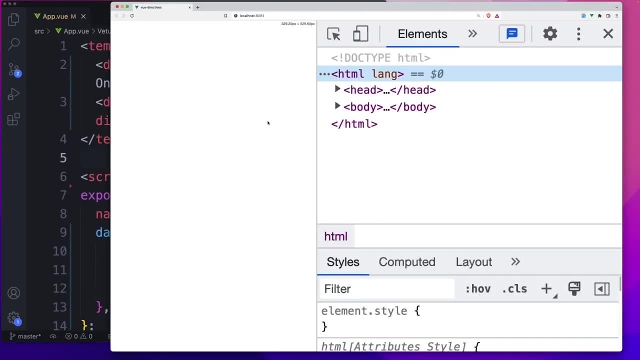 if i right click here, go inspect. i'll scoot that across so you can see it inside of our app, right there, element one, which is our v show, that's still on the page, whereas element two is no longer there. if you're going to repeatedly toggle an element, i think v show is the better. 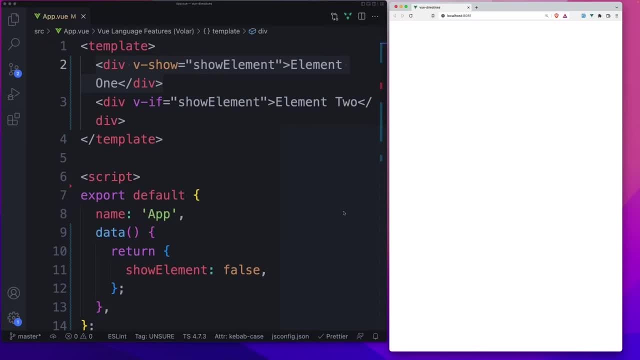 directive. if you're only going to determine on page load, or maybe even just once after page load, whether to show or hide an element, v if or v show, is fine. so a couple of things to point out here. don't use v if and v4 on the same element. now we haven't covered v4 yet. that's coming later in this. 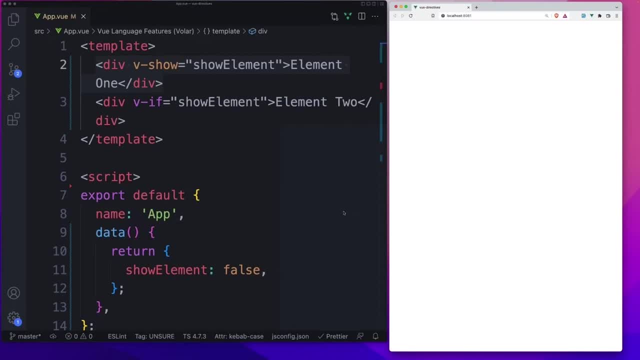 video. but if you do do that v if has a higher priority. and then, lastly, where you use v else, that has to follow in terms of the html structure, your vf. so in this example, here, this will work correctly. but if i try and place it in the same way, i'm going to use v if and then i'm going to. 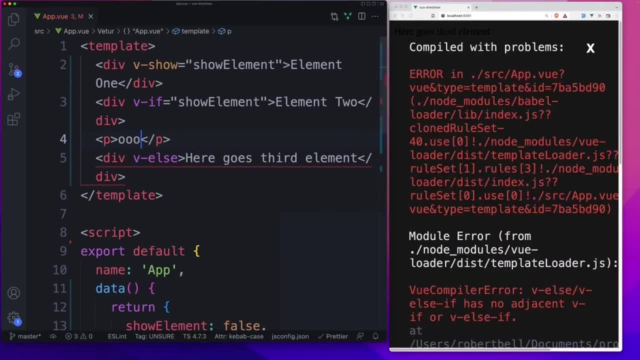 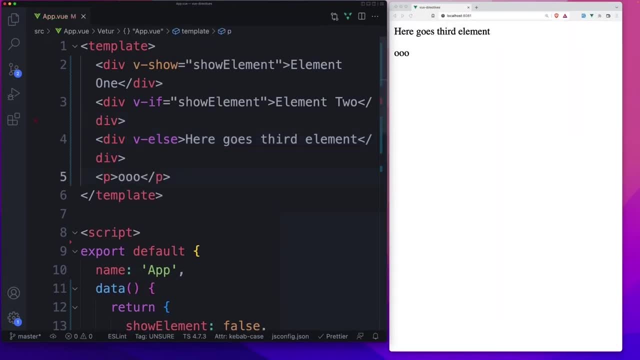 use v on if, but if i try and place a paragraph tag between these two, you'll notice we get an error and my editor doesn't like it, so you can't have that. you could have that coming after the vls and that's going to work fine, and the same would go if you're using v else. if. 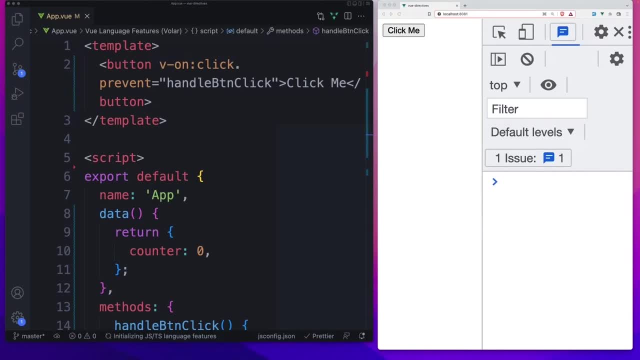 okay, we can move on now and our next directive is the v on directive. now vian should look familiar to you. we've just covered it in the usage section of this video, but we use vion to add eventlessness to our elements, so in the button on screen we're using von. 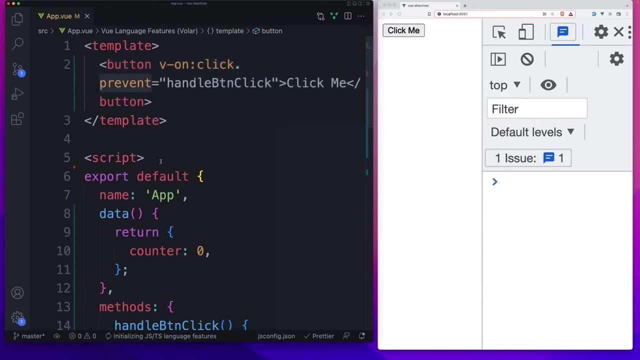 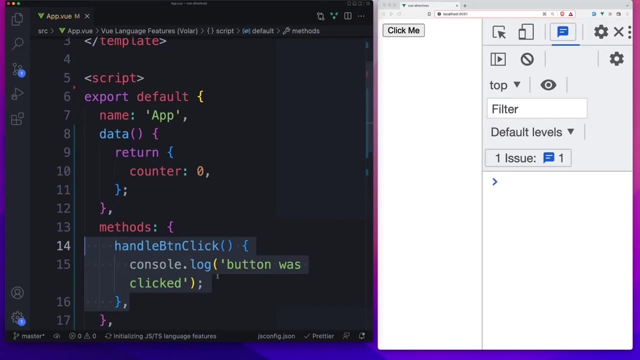 to add a click event. we're also going to use the modify prevent and on click we'll call the function handle button click and it's right here inside of my methods and all i'm doing is console logging out. button was clicked, so we click it and in our console we get button was clicked. 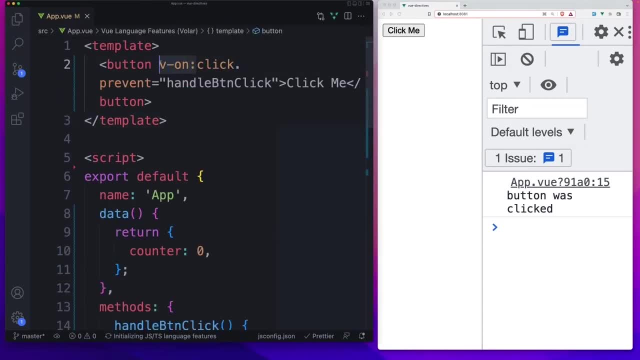 and we do have a shorthand for vion. so we can get rid of all of that and we can replace it with the add symbol and that click argument that we're passing in right there. that's your javascript event that you're looking to add. so click, blur, mouse, enter, etc. now, in terms of 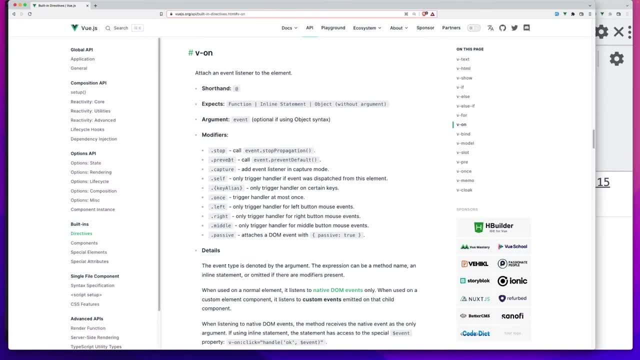 modifiers. we have a whole bunch of modifiers to choose from, so i've been using the prevent modifier, which is effectively eventprevent default. but you've also got stop capture self. you've even got left, right and middle, which only triggers the handlers for the left, right and 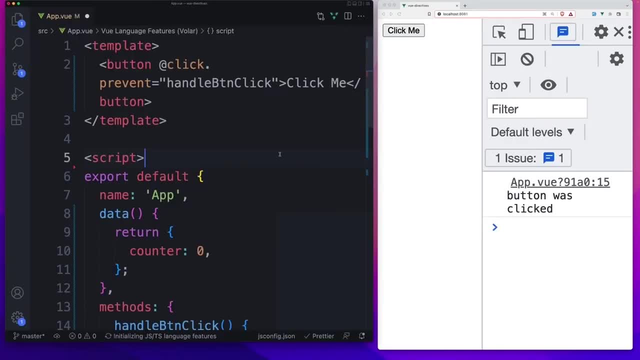 middle button mouse events. you can also pass in arguments into your function. so if you wanted to do that, just add in your parentheses and then press enter and you're good to go. so now let's pass your arguments in, and in addition to your own arguments, you have access to the special 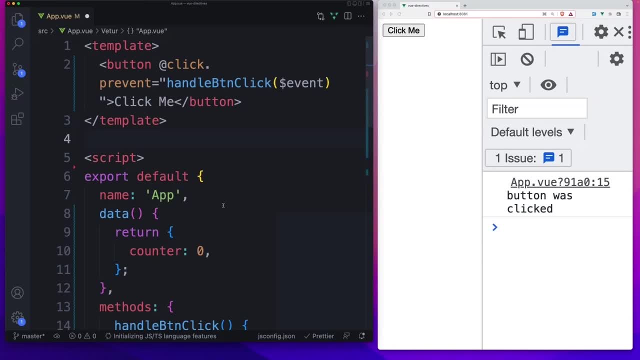 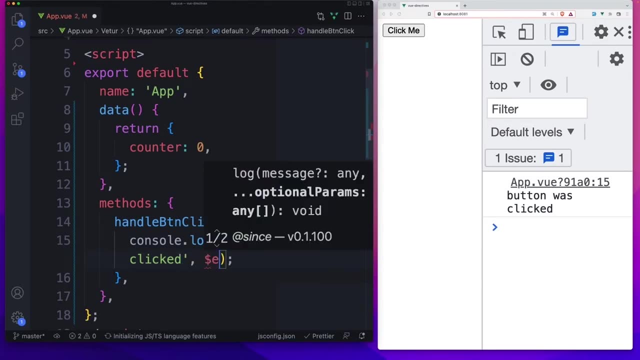 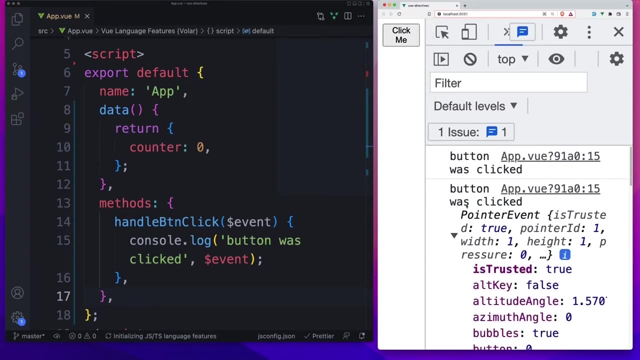 dollar sign event argument. and that is as you'd expect from normal ad event listener. that gives us access to the event. so let's pass that in right here and then i'll console log it out and there you go. there's, our button was clicked and there's our event. now you don't have to pass. 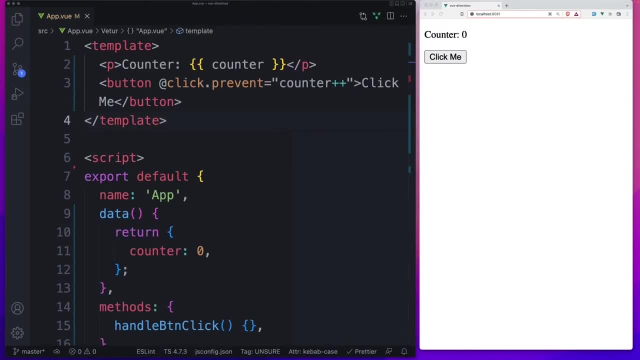 a function into your v on directive, you can also execute basic directives and you don't have to pass a function into your v on directive. you can also execute basic javascript. so i've set myself up here with a data property called counter, set to zero, and we're. 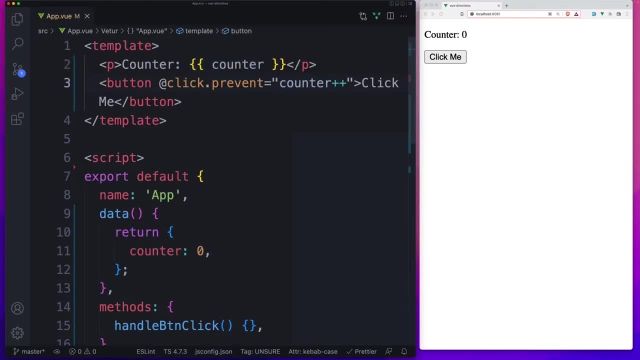 outputting that counter and on click we'll increment our counter. now we don't need that anymore, so let me get rid of that. okay, when i click there, you go one, two, three, four. now you could also have just called a function there and then done that same thing inside of your function. 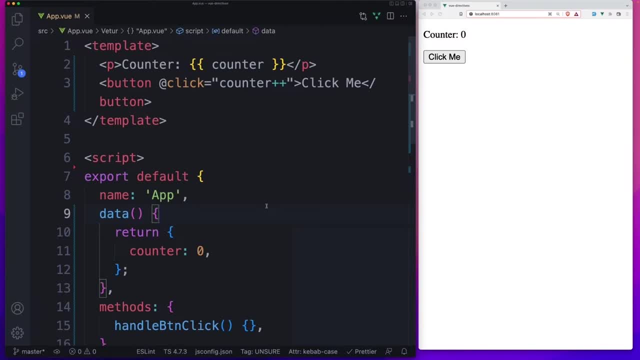 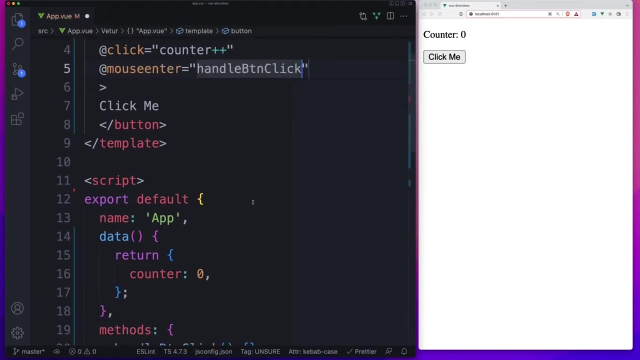 what if you wanted multiple v on directives or multiple directives on the same element? so let me just make this a little bit more readable. so, on click, we'll increment our counter, we'll leave that the same and then let's target it to mouse enter and let's just call our handle button click function that we've already got set. 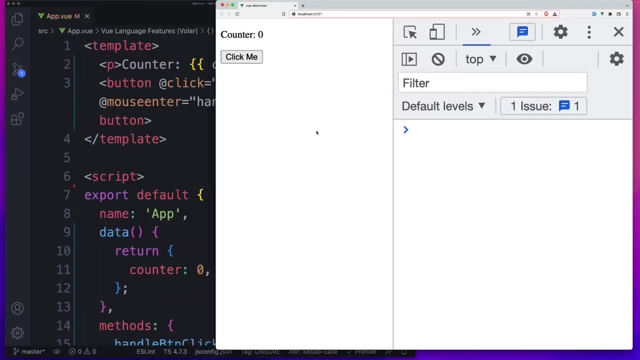 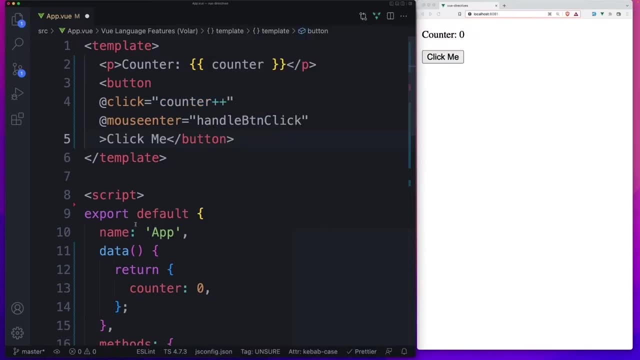 up and inside of that we'll just console log hovered. okay, i'm back in our browser now. when i hover, we get the hovered in a console log and when i click, the counter is incremented. now, personally, i prefer this over here. for me this is just more readable. however, you can combine your v. 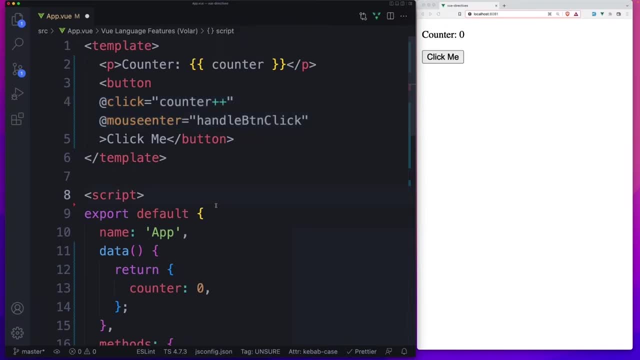 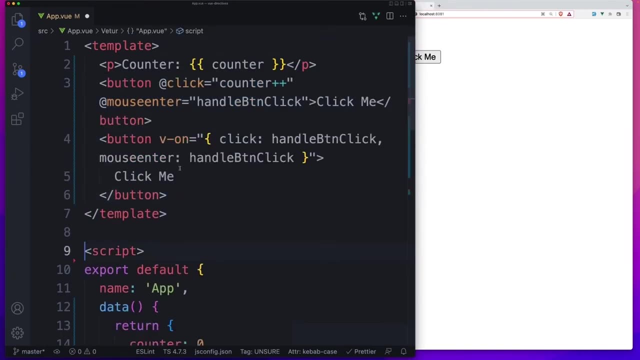 ons into the object syntax, but there's a few things different about it. so what, we've got over here with our two v under directives. we could write something like this: so we start off with v on, then we have our equals and our two quotation marks, and then we list each of our arguments paired with our functions. 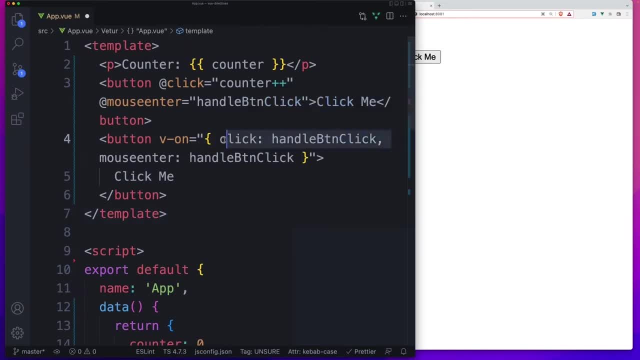 or our method that we want to call, and these are comma separated. you can have as many as you want inside of these brackets, but the thing to note here is that with this object syntax, we do lose the option to use modifiers. and, last but not least, you can emit events between components. 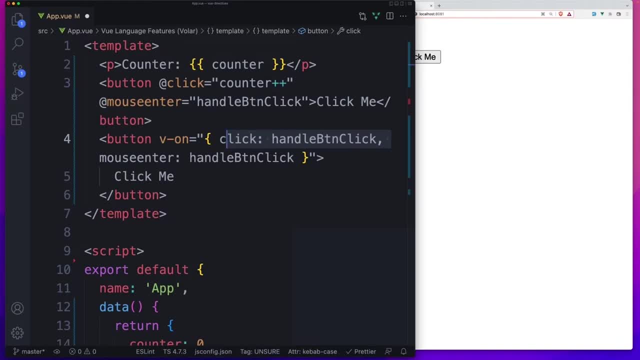 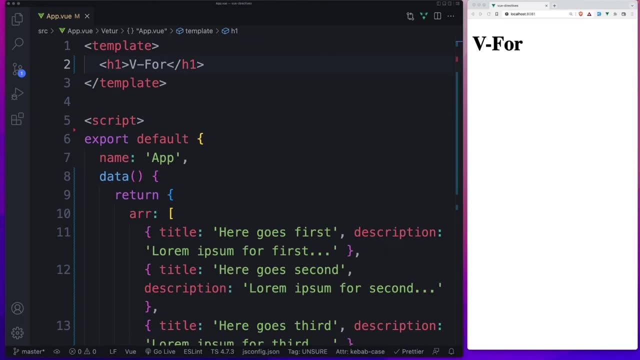 but i'm going to be doing a separate component video, so i'll leave that subject for my components video. now, one of the things that you're going to do a lot in any application is look to iterate over data. for example, you might run an api call. 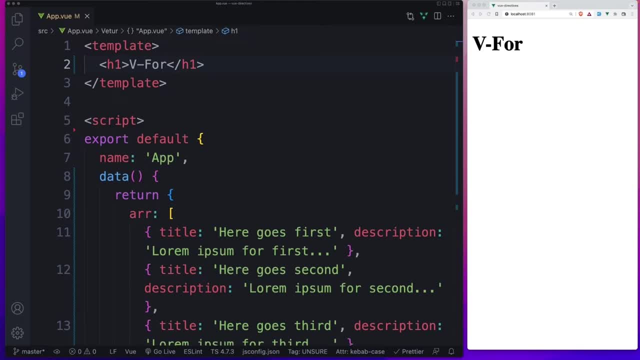 get some sort of data back, say your blog posts, and now you need to output that. so our next directive, v4, allows you to handle those circumstances. using our v4 directive, we can iterate over your typical array and objects, but then, in addition to that, numbers, strings. 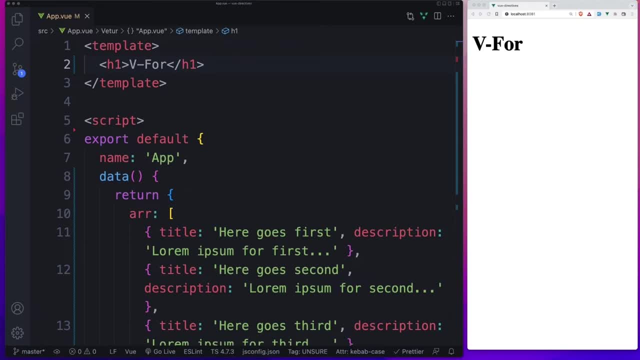 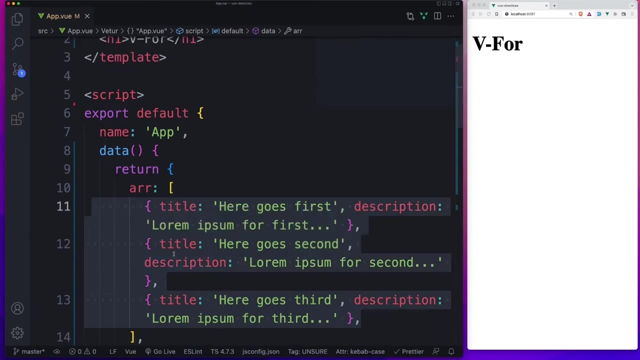 and values that implement the iterable protocol. so think javascript, maps and sets. so let's start off with our first example here, going through arrays. now i've set myself up with an array property and all we have is a title and description and there's three objects inside of that, so we need to get this now on our page. 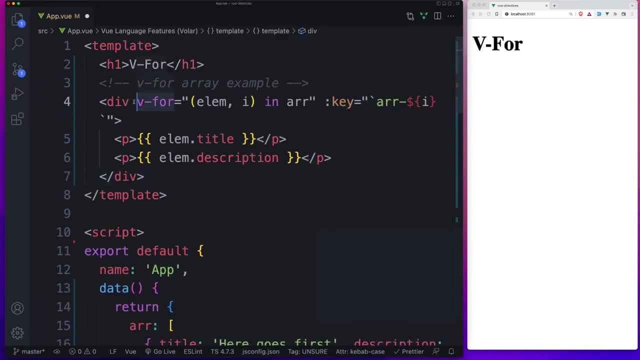 with as little code as possible, right? so the first thing we do is we start off with our v4- there's no shorthand for this- and then we can reference it by whatever name we want. here i've called it lm, and we'll use that inside the loop itself to access the properties. you can also get access to the index property. 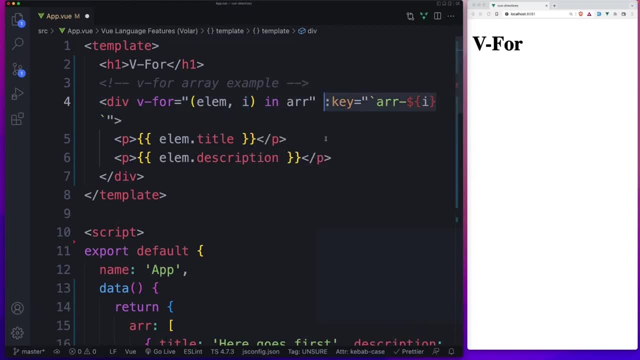 which i'm using to assign a unique key. so one of the things that view looks for when you set up a view for is some sort of unique identifier that makes it easier for view to update that particular element. and what i'm doing here is i'm using vbind, which is going to be the next directive we're. 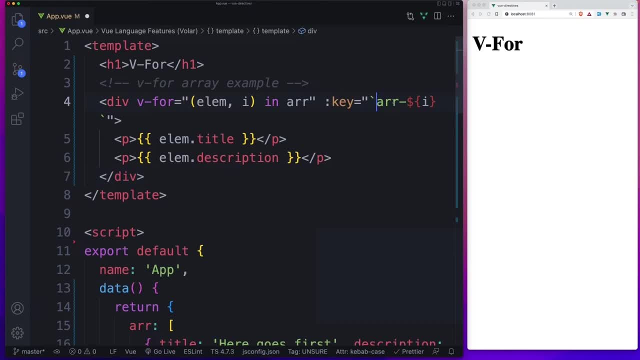 going to look at, and then i'm using template strings so that i can have a combination of what we want to set up specifically for the index, as well as, of course, the index. so that value, right there is what i'm placing in there now. most of the times, when you get back an array, 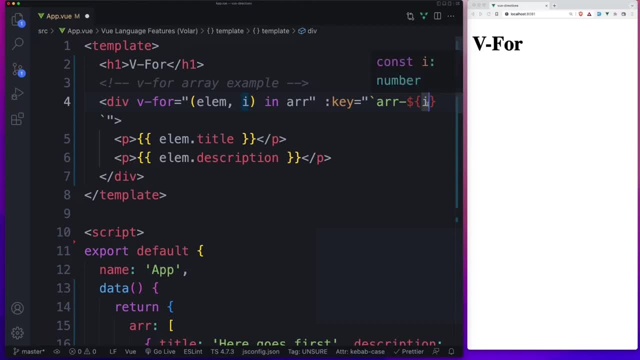 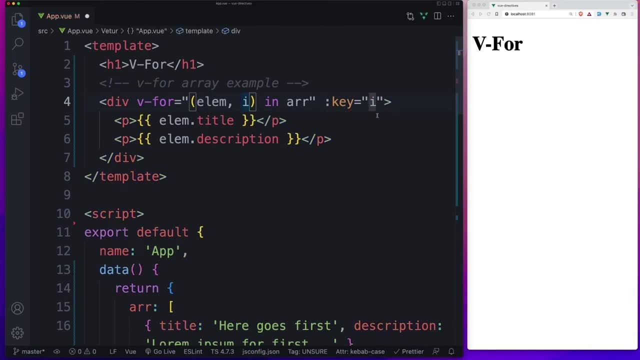 from your api call. you'll have an id, so you don't need to set it up the way i have here, and you could also just have referenced the i value like that. the reason why i do it the way i've done it is just to make sure that that key value is truly unique on the page. so here's our v4, which is that: 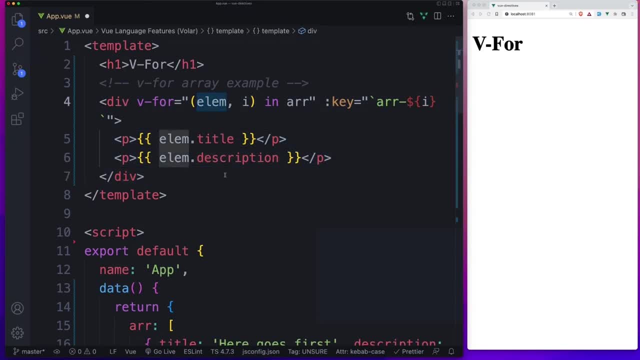 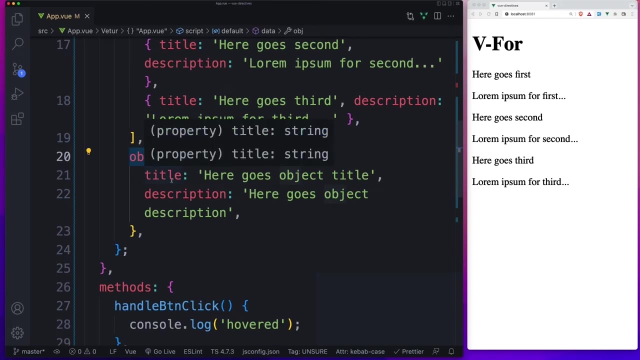 development there, closing off, and then inside of that, to this element property, and that gives me access to the title and the description. so let's save that and on our screen we can now see our v4 output. all right, let's move on to looping through objects. so i've set myself up with a data object property with two properties: title and description. 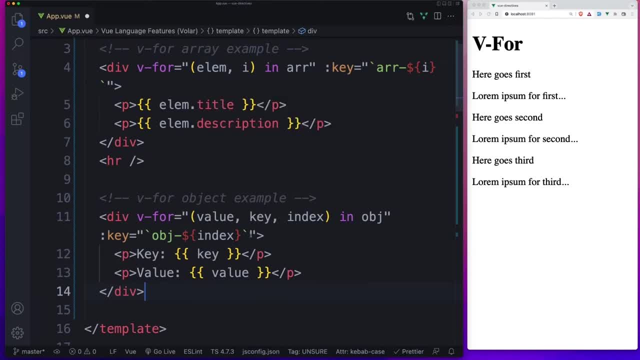 so using the same v4, just like we did with the arrays, but we need an extra parameter now inside of our brackets. so we've got value, key and index and then inside of that loop, i'm just outputting the key and the value. we'll save that and on our screen, there you go, key value, key value. now you. 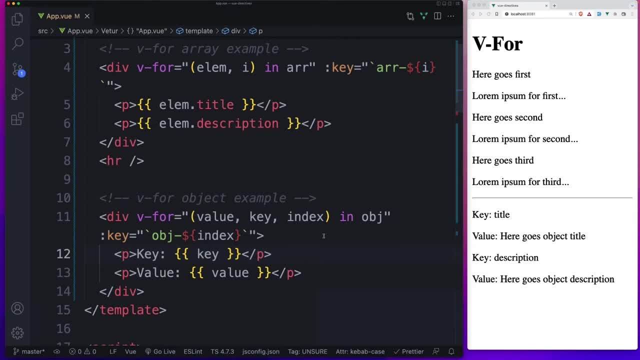 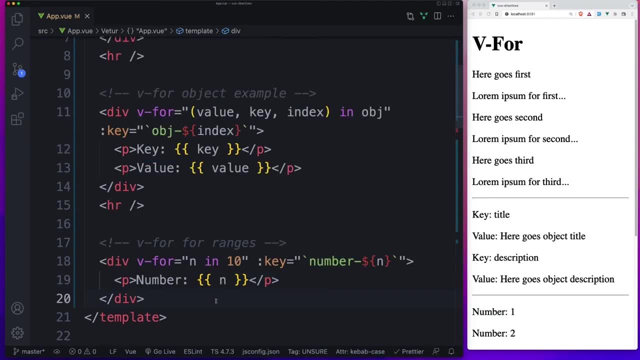 don't just have to use v4 for objects and arrays. as i've already mentioned, we can also use it just to loop through, say, 1 to 10.. so i'm going to set up a very quick v4 here which can cycle through from 1 through to 10 and i'll output that number inside of the loop and there you have it on the 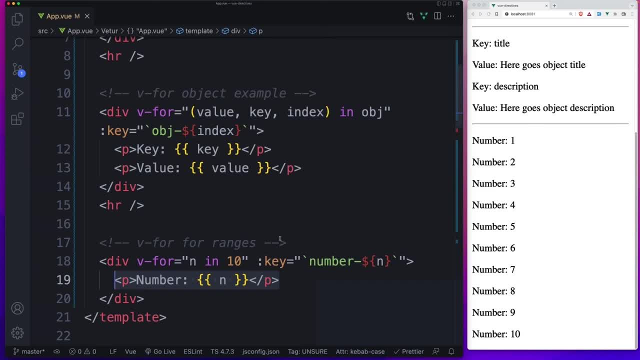 screen. there numbers 1 through to 10.. now, as i pointed out in the v if directive, just be careful not to use vf and v4 together. if you use vf and v4 together, just keep that example in mind in the video and i'll show you how to add that later in the video. so, without further ado, i'm just going to. 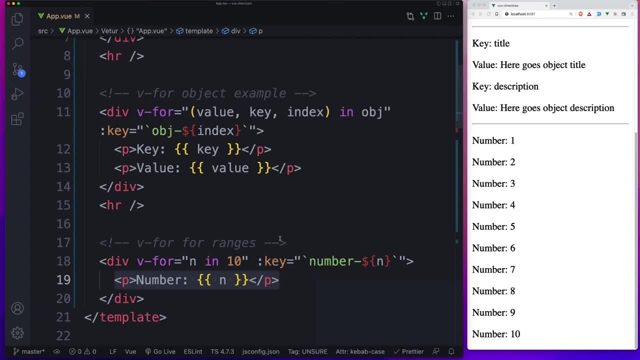 now, as i pointed out in the v? if directive, just be careful not to use v, if and v4 together. if you use a If you do, VF takes precedent and you won't get your V4 output on the page. The last thing to point out is that you can nest your V4s inside of them. 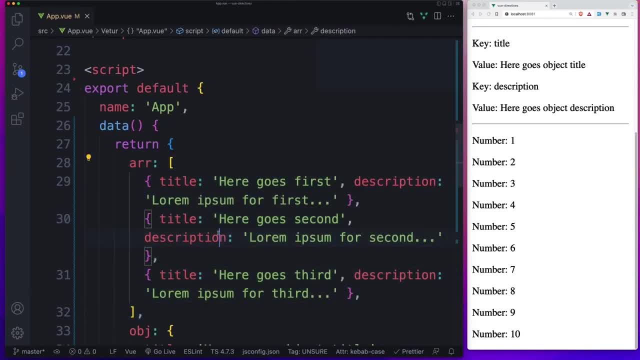 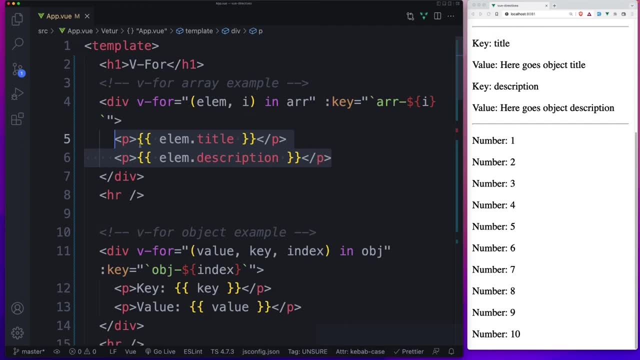 So let's imagine this array that I'm outputting over here had a further property that in itself was an array Inside of my V4. for the array right over here I could just run another V4.. Now we come to VBIND, which for me is a directive that I think you'll use most often. 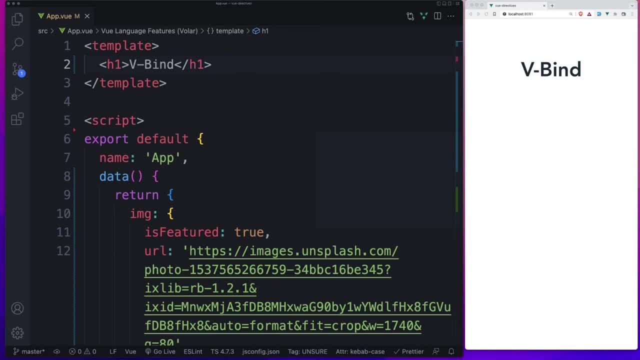 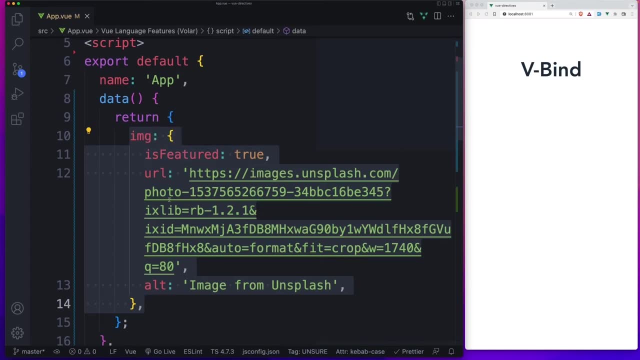 VBIND gives us one-way data binding. So what do we mean when we say one-way data binding? Well, we've got this image property inside of our data section and that gives me access to three further properties: isFeatured URL and alt. 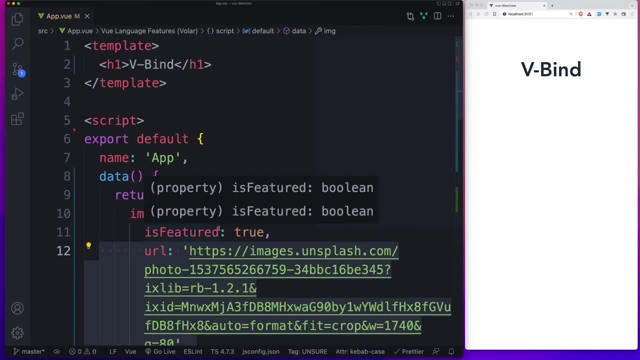 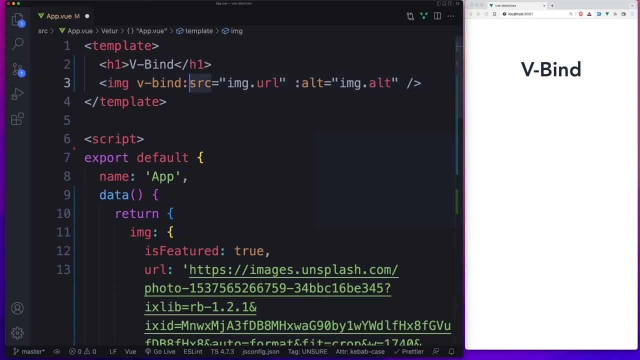 So, to begin with, I want to output this alt and URL inside of my template, and that's what I'm going to use VBIND for. So we start off with V-BIND and then we pass in the attribute that we're looking to bind. 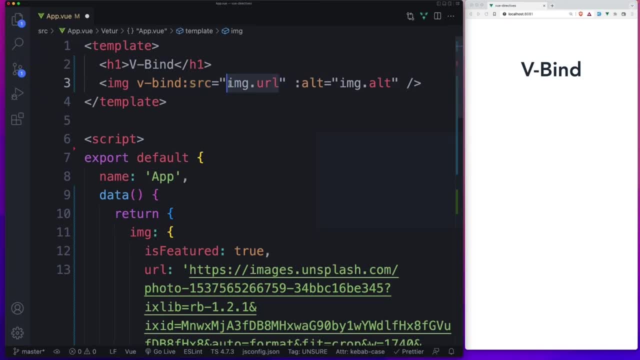 to. After that. the value we're passing in is the property that we want to output. So imageURL. is that one right there. image and then URL. Now VBIND also has a shorthand, and that's the shorthand version, right there. 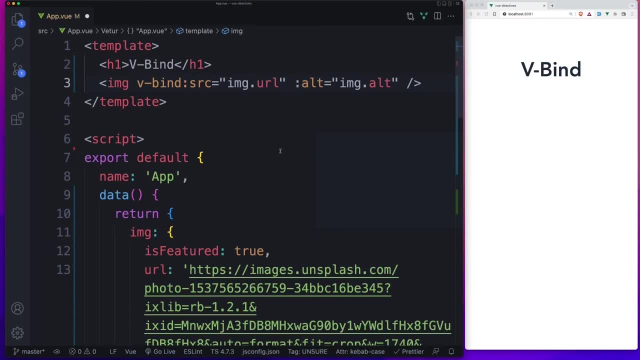 And again, as with all of these shorthands, either or is fine, but just be consistent throughout your application. Personally, I tend to use that shorthand version there, And you can also use VBIND for props, but I'm doing a separate prop video for that. 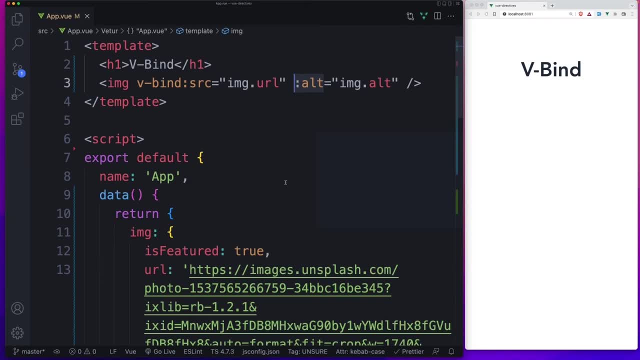 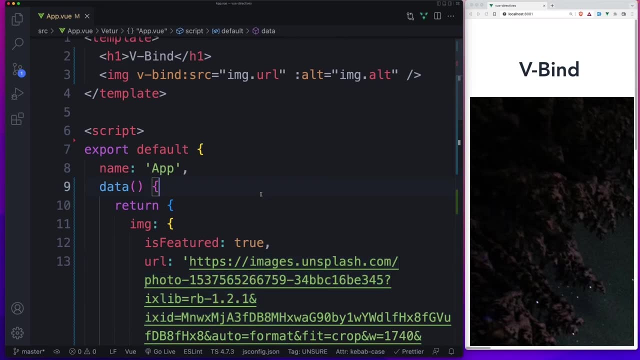 so I'm not going to touch on that in this particular video. So let's save that and see what we get output. Great, So there's our image. that's just a random URL I'm pulling in from Unsplash. Now the problem we can see straight away is that this image 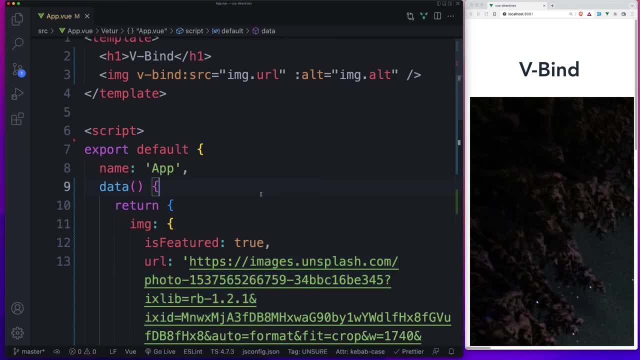 This image is too large, So we could modify the style ourselves, but we could also use VBIND for it. So just like we can bind to the SRC and the ALT, we can also bind to the styles for this element. So in this instance, right here, I'm using the shorthand version. 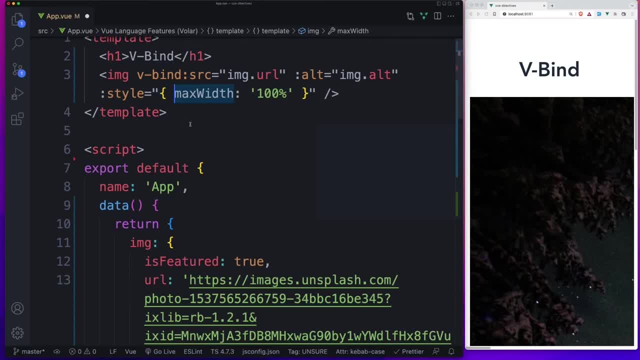 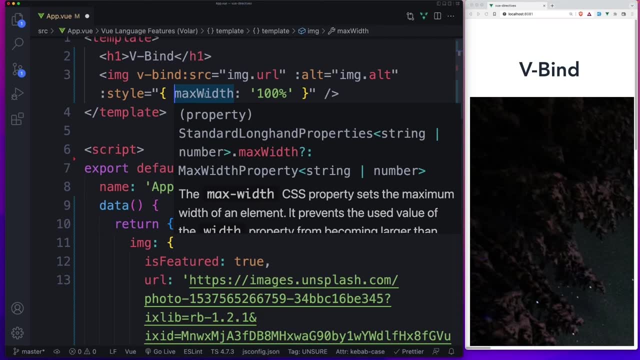 So we need our object syntax and we're passing in max width, which I want to be 100%. Now note: this is CSS written in JavaScript. So where you do that, you'll typically write camel case for What would be that, right there. 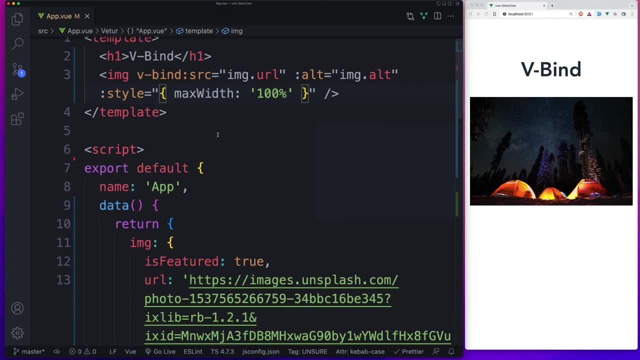 If I save my changes, now we have a max width of 100.. Now this isn't really very real world, right? You wouldn't do that. You could just. if you really wanted to do that, you could just do something like that. 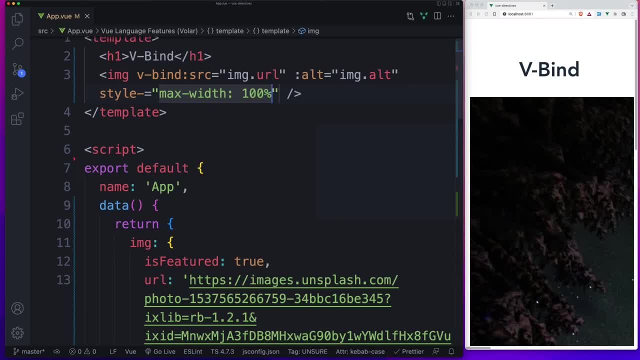 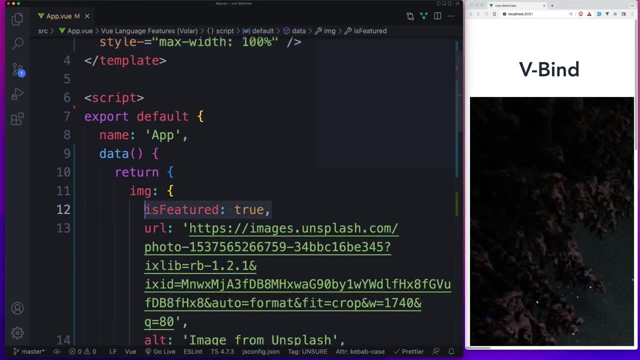 And, of course, you're going to get the same thing. So a more common use scenario is to assign a class dynamically. So let's go back to our image property. We've got this isFeaturedTrue right And I've set up inside of my CSS. globally, I've set up a featured class. 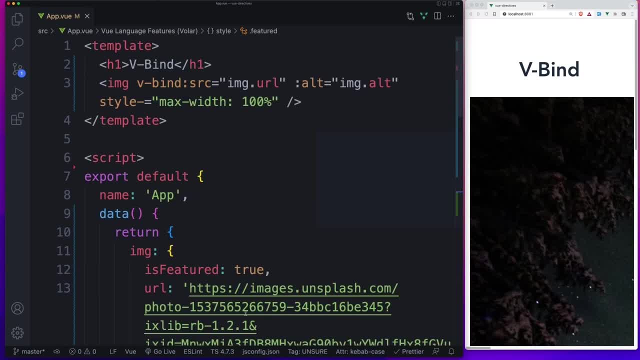 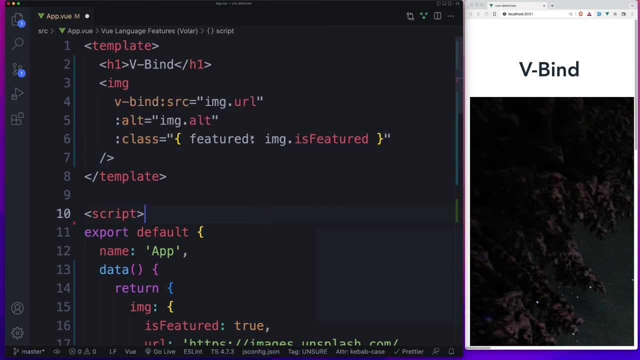 Which will set the width of 200 and give it a border of two pixels blue. So we can change what we've got over there to something like this: We can bind to the class attribute And then what we're saying to view is assign the class featured. if this expression is true, right? 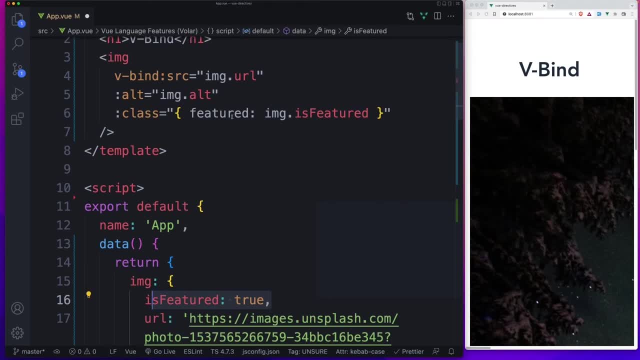 So imageisFeatured? well, that is true. So the class featured gets added to our image. We'll save that Great Now if we change this to false. and now we lose that right Because imageisFeatured is now false. 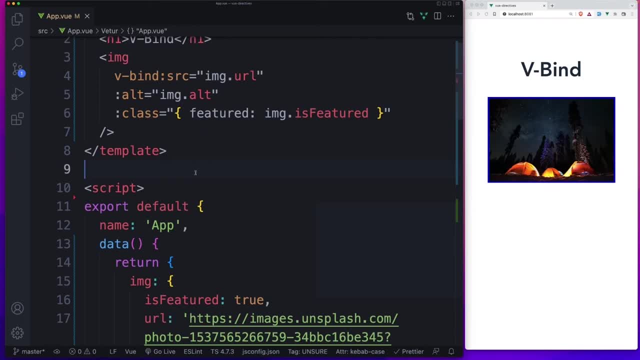 Now, this is just touching The surface of VBind. My advice is: go open up the VDocs and read through all of the stuff you can do, Particularly when it comes to style and class bindings, Because you can get very creative with how you assign your different classes and styles for your elements. 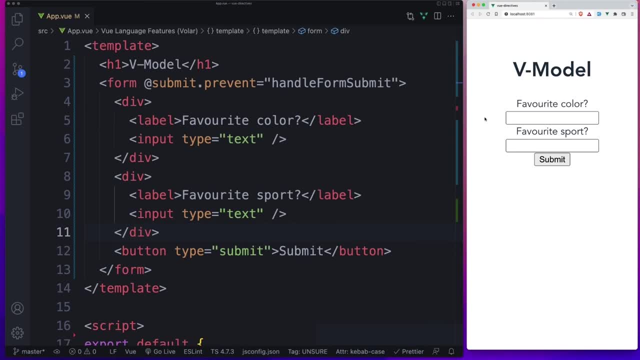 So we come to the last built-in directive that I'm going to look at in this video, And that's ViewModel. ViewModel gives us two-way data binding. So in our previous directive we touched on one way which was binding data from our application to elements on our page. 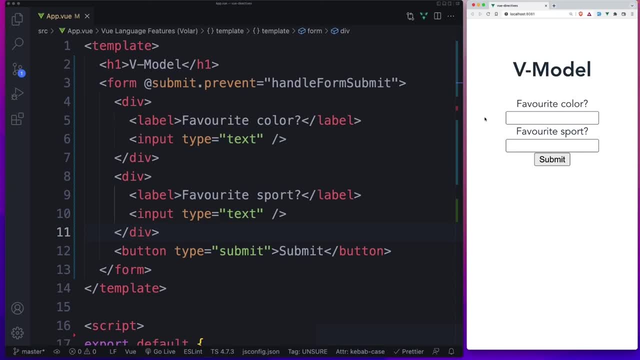 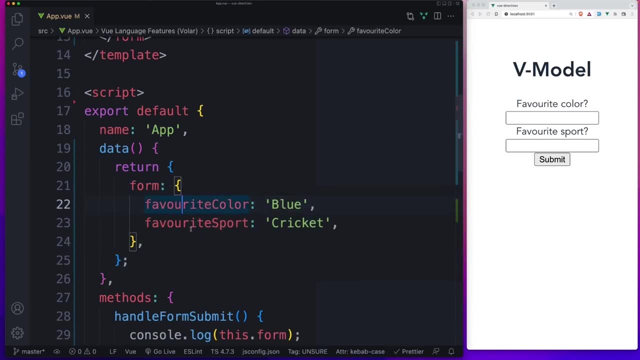 Two-way means we bind that data, but we have the ability to then update it. So let's look at what we've got set up here. I've set myself up with a data form property and that contains favorite color and favorite sport. 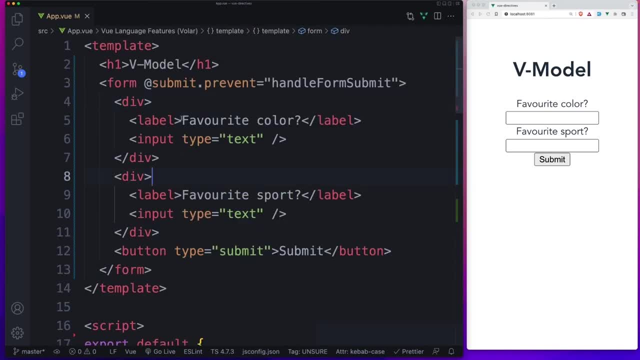 And inside of our template we have a basic HTML form And I'm also using our Vyond directive to add an event listener for the submit event, making sure we prevent defaults and then calling handleFormSubmit. So if you did watch the part of this video about the view on, this will all look familiar. 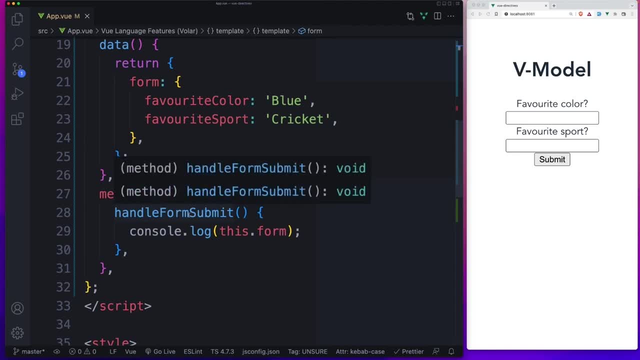 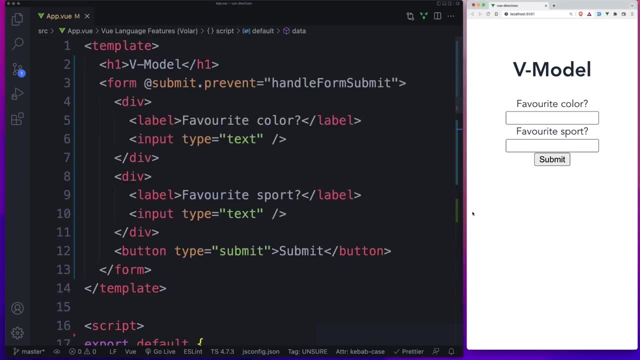 So that's exactly what we did with the button And then on our handleFormSubmit, I'm just going to consolelog thisform, which is that form right there. So before we make any changes, let's just see what we get by default. 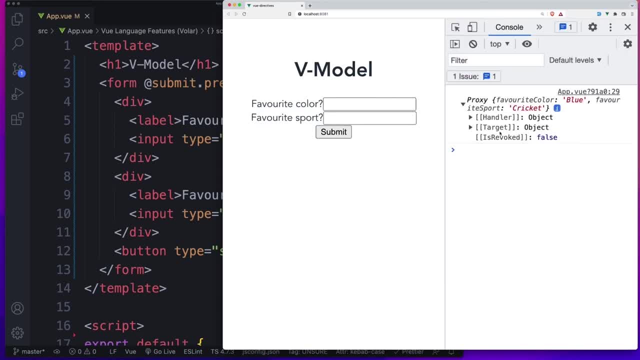 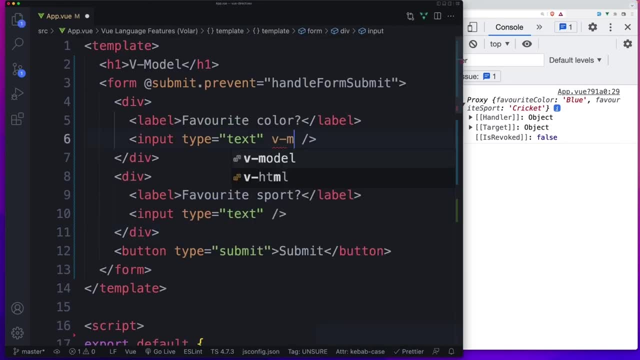 So I'll open up my inspector, we'll submit it and that's what we expect, right? Blue and crickets. We go have a look at our data. blue and crickets. So let's bind this now using ViewModel, So V-model, and we don't have any shorthands for this, so you're always going to output ViewModel. 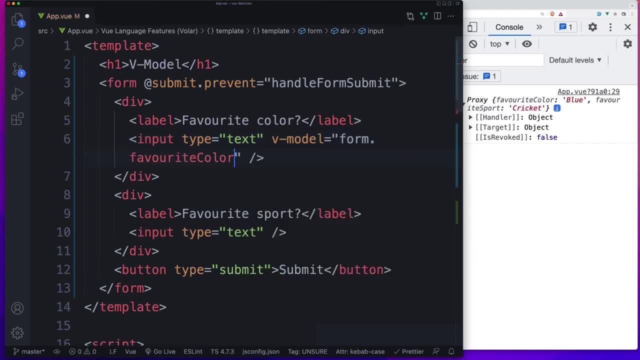 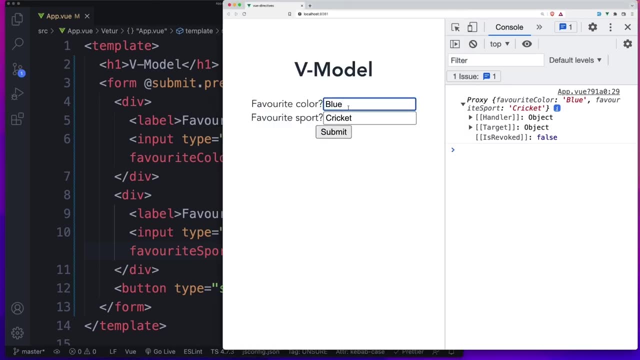 And then it's what you want it to bind, So formfavoriteColor, And we'll bind the bottom one for favorite sports. And now on the front end, now we've got those values pulled in. So so far that's one way. 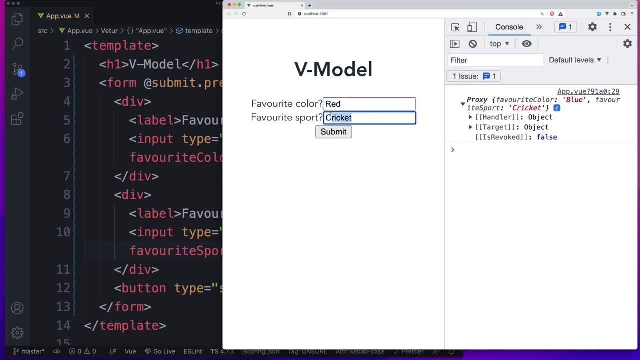 Now here's the two-way binding. Let's change this to red and we'll change this to rugby. And now when I submit that form, color red, sport, rugby. So the typical way that I'll use ViewModel is, say, registration forms, login forms, user profile forms. 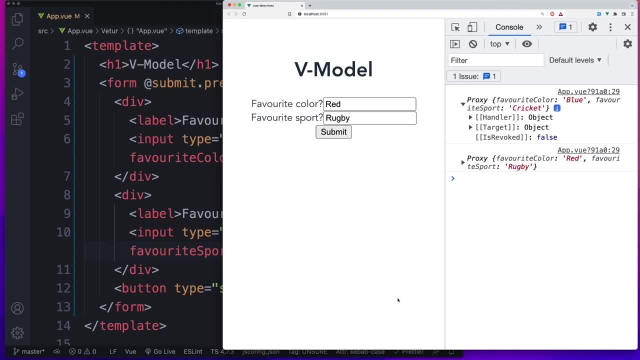 anywhere where you either want the user just to enter that data from scratch, or you want to show them starting values, but allow them to edit that data and then submit that. Now there's one important part about this, which is that you can also use V-bind with your components and props. 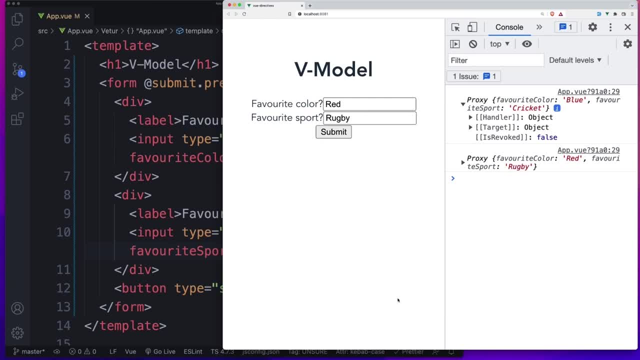 But again, I'm doing a separate video on components and props, So I'll be sure to cover that subject in most likely both of those videos. And the last thing to point out is that there are a couple of modifiers that you can use. 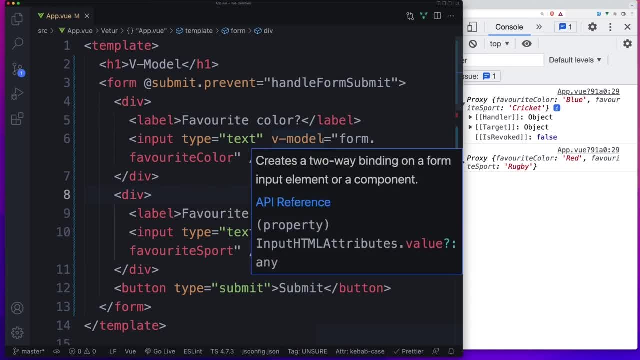 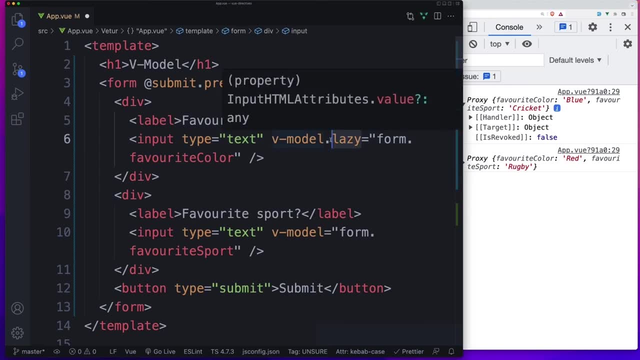 So on our V-model we can use lazy, So lazy will only listen for change events Once the user has completed their update. so the change JavaScript event rather than the input event. You can also cast the value to a number and then you can trim it as well. 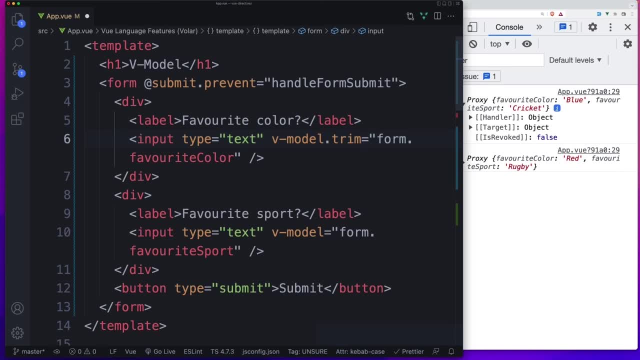 And that's everything that I'm going to run through in this short video. Now, these are not all of the default view directives, So I encourage you, open up the view docs, have a look through at some of the lesser known ones and have a play around with them. 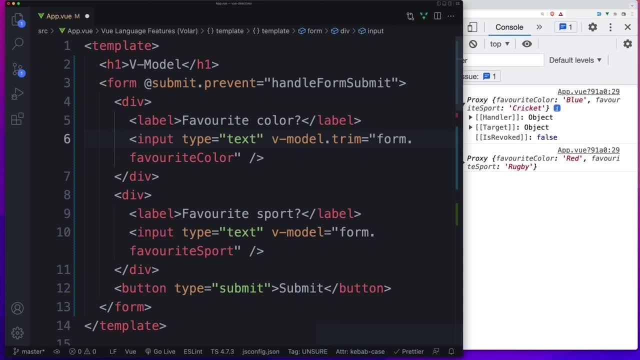 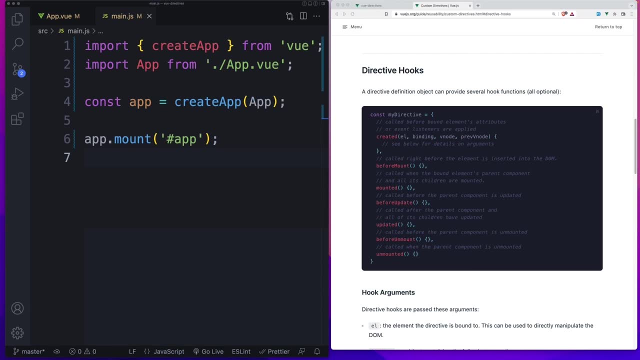 But what happens if you need something more, if you need a custom directive? To finish off this video, we're going to write ourselves our own custom view directive. Now, if you're someone who's just learning the basics of view directives, then obviously the first thing for you to do is to master the built-in directives. 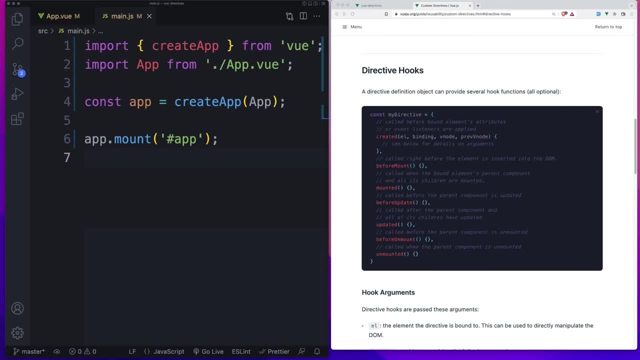 And that's why the majority of this video I've focused on that, But I do think it's a good idea just to understand a few of the concepts around custom directives. So we're going to keep it very simple And I'm only going to create a very, very basic example for you. 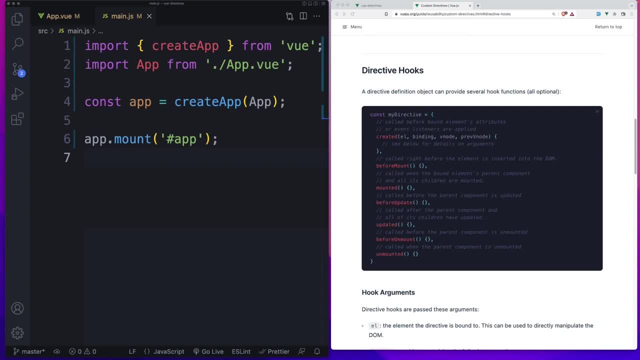 So that later on, once you're happy with the built-in directives, you can return to custom directives, And I'll be doing a separate custom view directives video where I'll go into more details about all of the various points around it. So the custom directive that we're going to create here is simply going to make 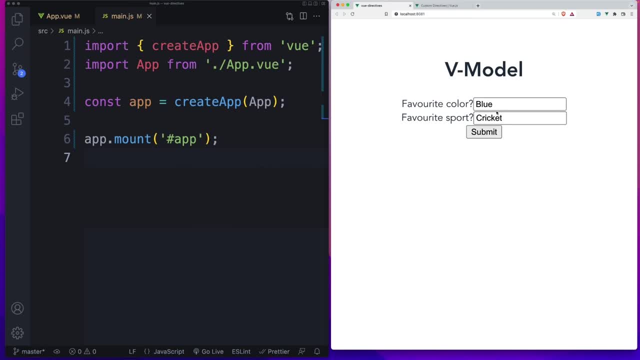 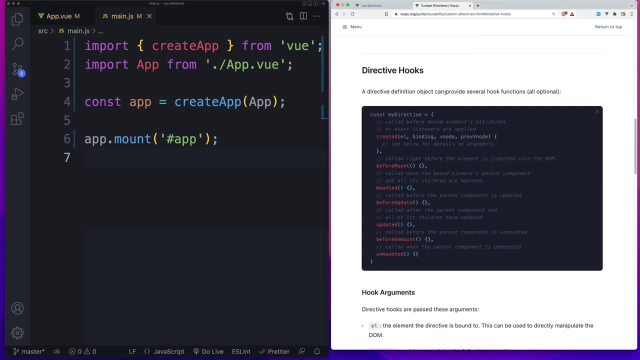 the form input from our previous directive focus on page load. Now, to do that, we need to first of all tell Vue which hook we want to use. So in front of you here we've got all of the various hooks available to us in Vue 3.. 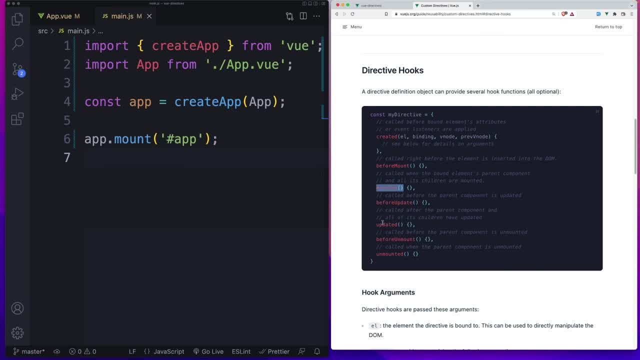 And we're going to hook into the mounted option right here Now. once you hook into that, you're going to see that we've got all of the various hooks available to us in Vue 3.. And once you hook into that, you then get passed in various hook arguments. 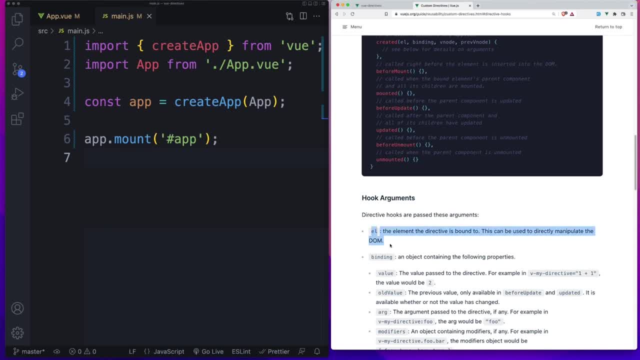 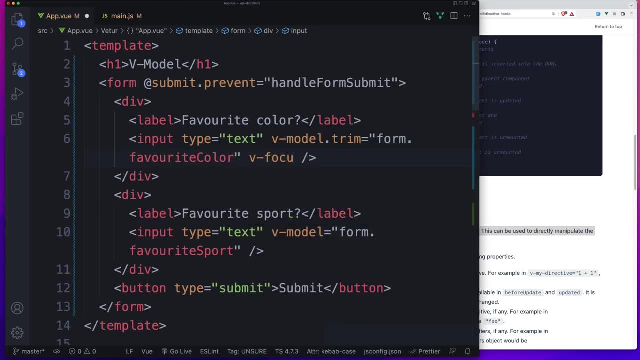 The only one we care about is the actual element that we're hooking into. So if we go back to our code inside of appvue, to this favorite color, I'm going to add V-focus. Now, focus is the name that we're going to use. 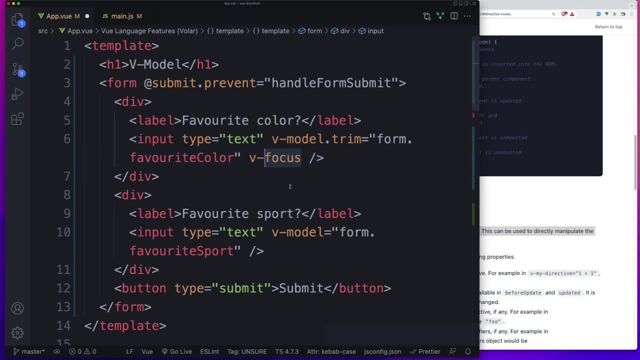 V, remember, is the prefix for directives that gets added on by Vue. Now that means, when Vue runs through our custom directive, the element that we get passed in is this actual input right there. Okay, Now I'm going to do this inside of my mainjs, where we run our create app.